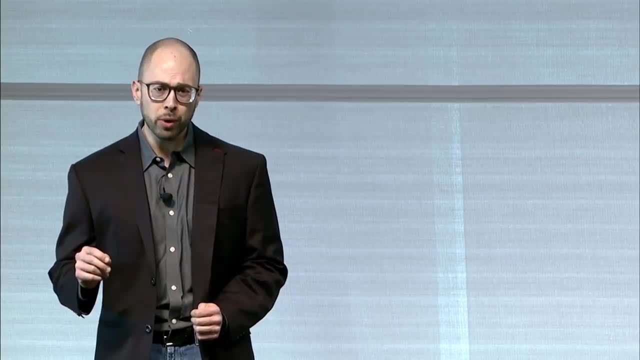 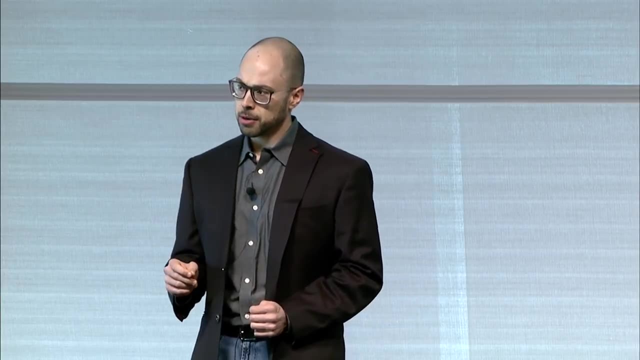 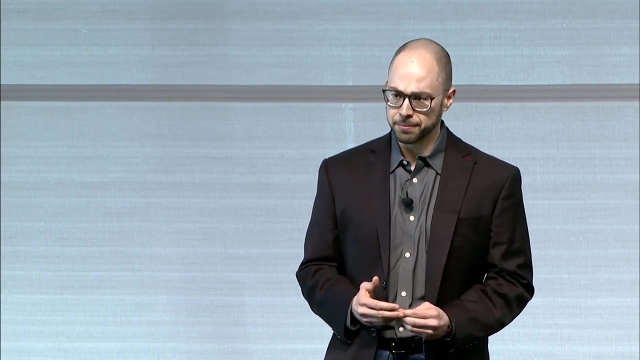 first or most conveniently located one. Where is the handle of that cart or basket? What additional moving objects do you have to be most mindful of? Other shoppers- Children, Dogs. This sounds exhausting, doesn't it? You can open your eyes For the 300 million who are visually impaired worldwide. this. 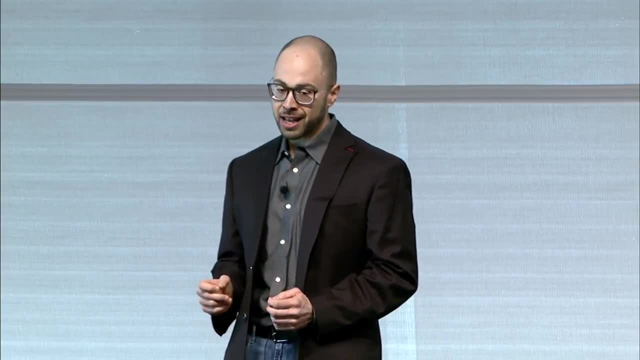 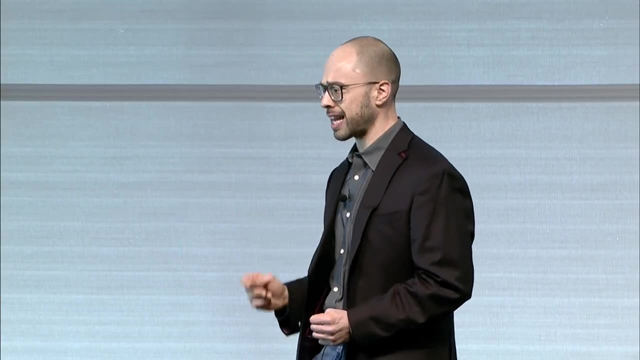 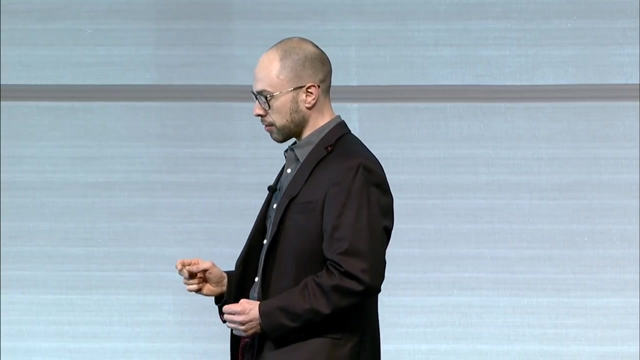 seemingly simple task is a complex journey fraught with challenges, And the anxiety you may have experienced by attempting to answer these questions doesn't come close to capturing how truly taxing and painful it is to navigate through everyday tasks. Most of us take for granted the ability of our visual system to spatially analyze the environment and the 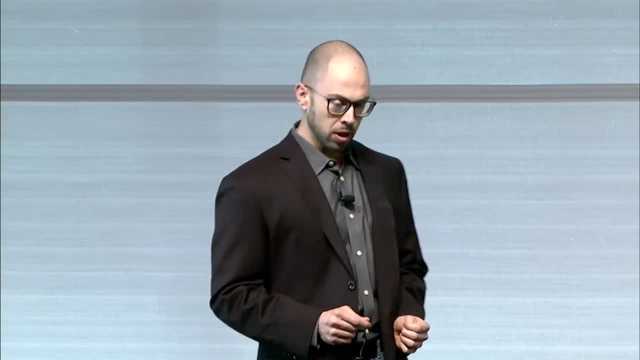 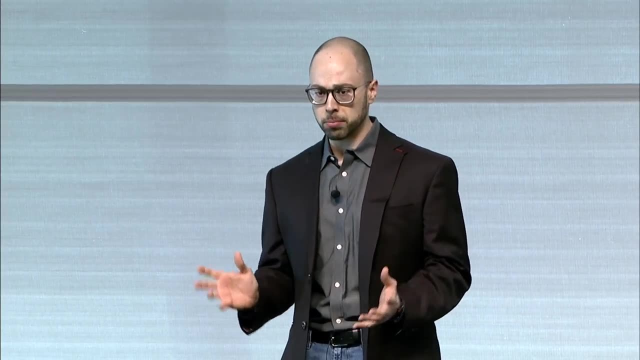 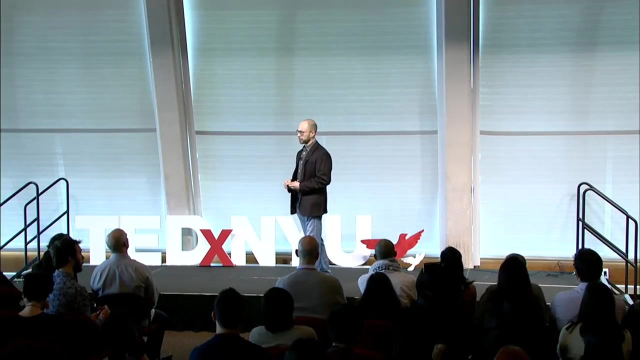 use of this information for seamless navigation. For the last 30 years of my life, I have watched my vision at the outermost extent in the periphery fade from clear to blurry and eventually to nothing, shrinking to a small tunnel right in the very center. I have a rare disease called choroideremia that has 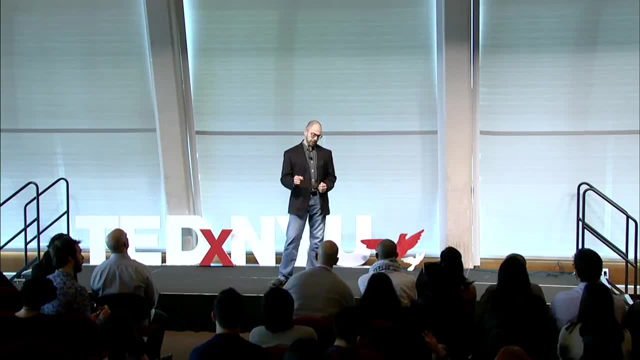 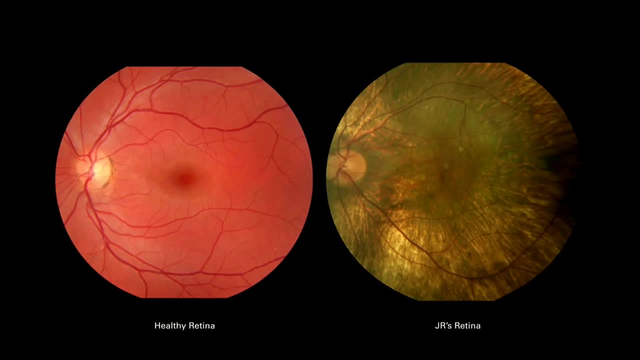 been robbing me of my sight since I was a child. Here is an inside view of a healthy retina and a side-by-side view of mine. Presently, I am legally blind and setbacks such as worsening vision, medical complications and professional obstacles have been the norm. 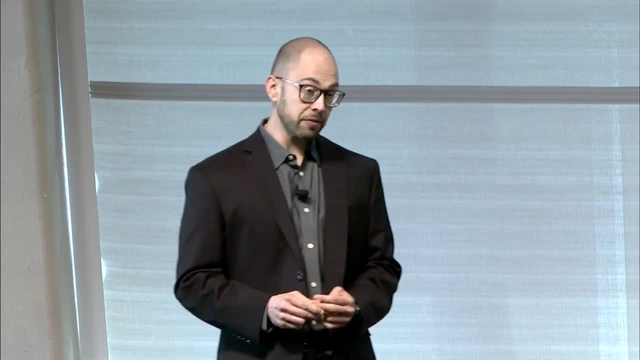 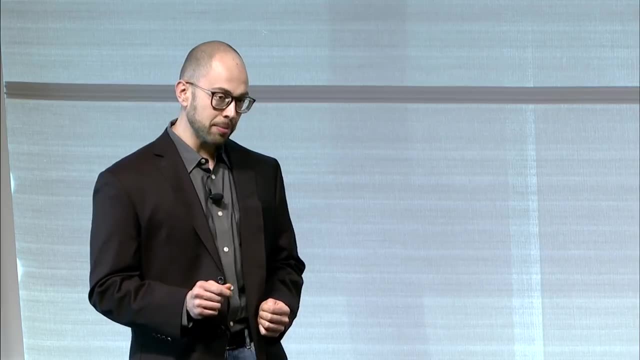 But the truth is I am also incredibly fortunate. I have an amazing wife who is the ultimate partner and aid. She helps guide me places, As a matter of fact, in dim light, when I am at my worst. we have our own hand-holding squeeze codes to signal ramps, curbs, stairs. 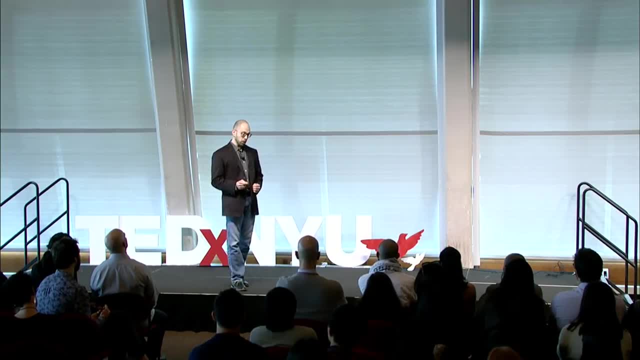 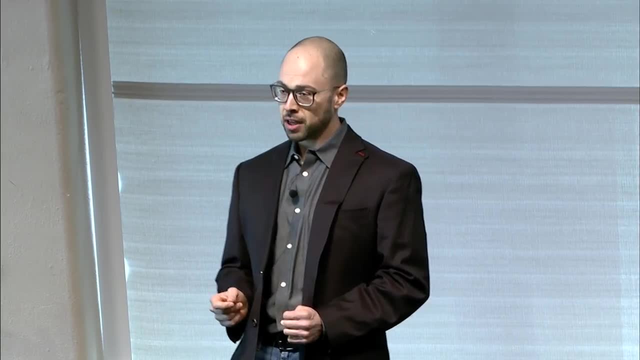 obstacles and occasionally even the irresistible pastry. Strong squeezes, light squeezes, sequence squeezes, squeezes in doublets, in triplets. there is an art to it. I have a strong family and very supportive colleagues and friends who are willing to help me. I have a strong family and very supportive colleagues and friends who are willing to help me. I have a strong family and very supportive colleagues and friends who are willing to help me. I have high standard personal and professionalی friends who are willing to lend me their 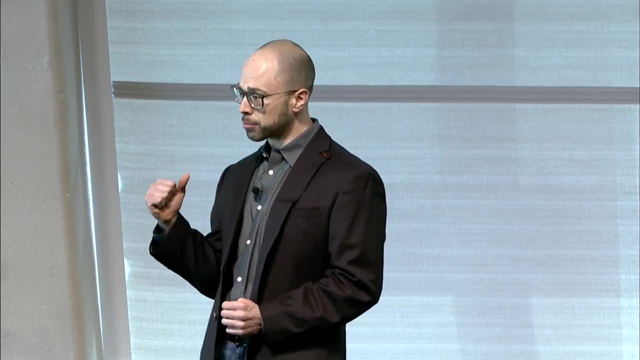 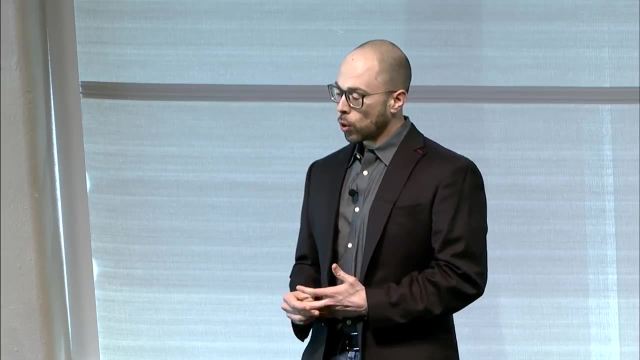 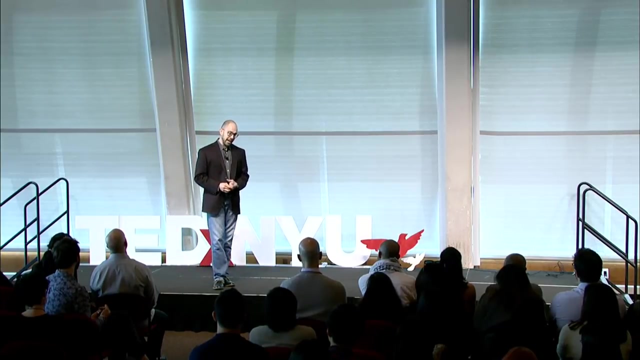 shoulder-arm, forearm or hand, guiding me like a train, cabooseragorated streets, conference venues with neverending hallways or in between meeting locations. To be blunt, I would not be here today if I had not been able to hitch rides. But it has not and is 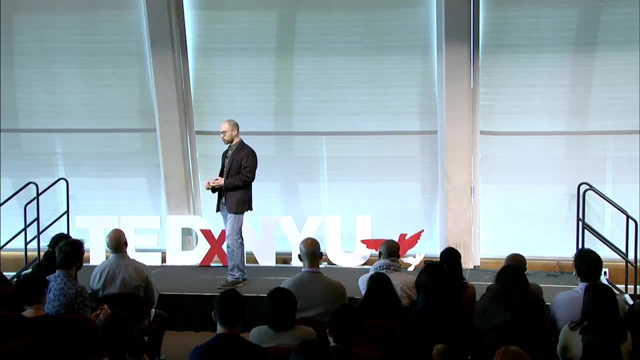 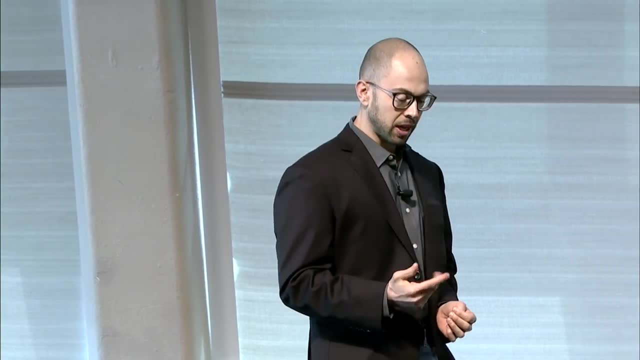 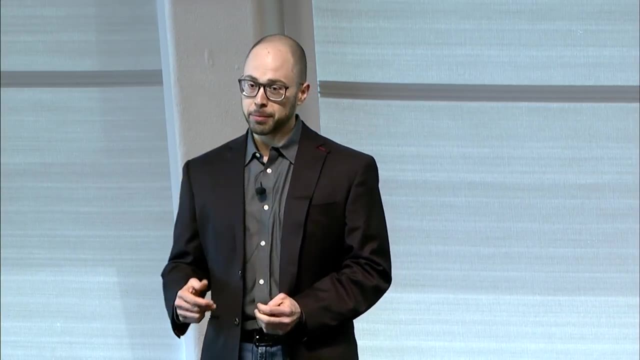 not always like this. I've been left out straight into danger and I wish certain periods of my life away. My visual disability has brought pain, but it has brought me tenacity, insight and opportunity. These gains have incrementally advanced every misstep, every stumble and every collision. 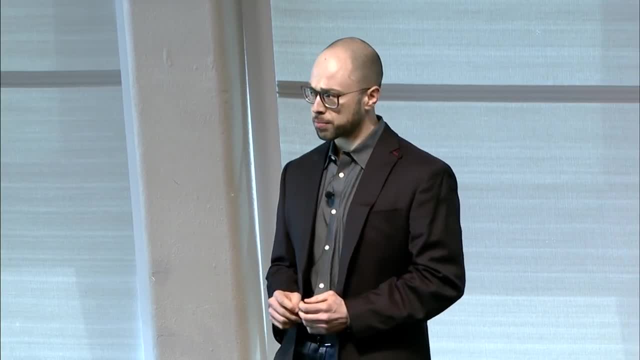 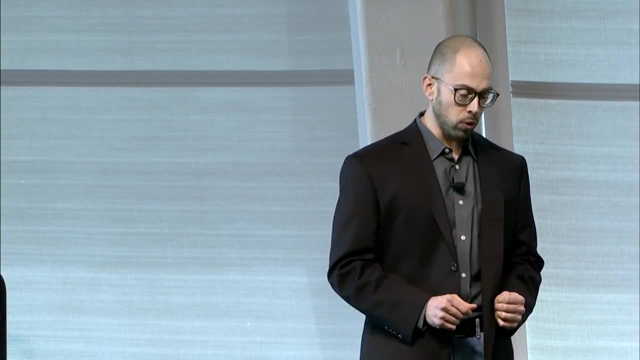 To be frank, I wish I could reverse my blindness and extend those improvements to those with vision loss across the spectrum. Presently, this is not an option. So how do we move forward? Well, every time I become increasingly frustrated with a situation, it's a deep breath, a reboot. 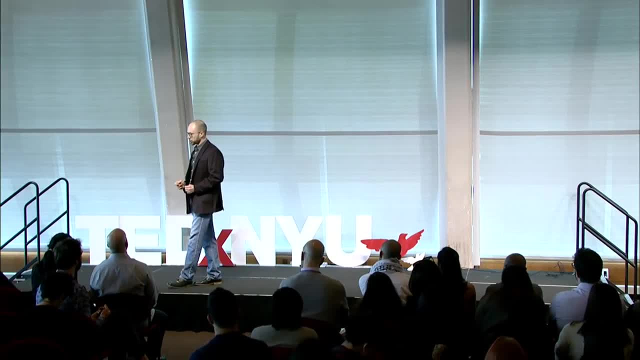 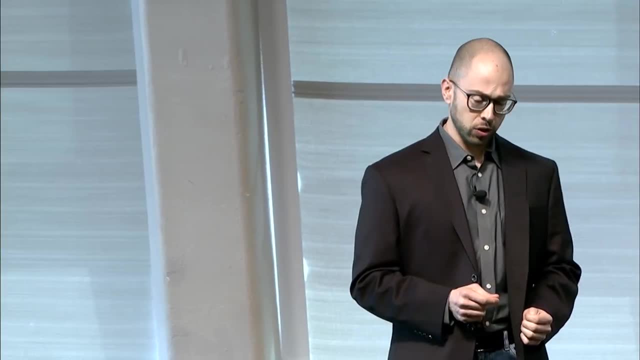 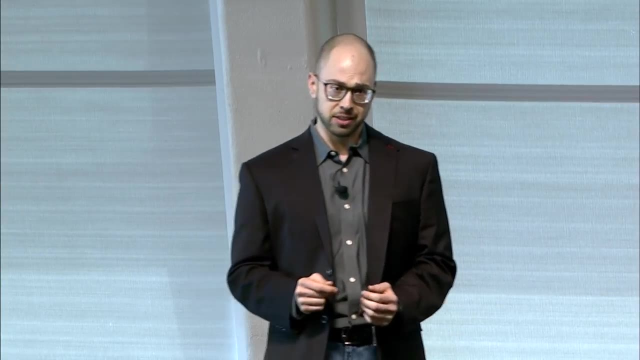 and an exercise in reframing. It's now a challenge: How do we fix it and solve or change the status quo to avoid these affecting circumstances? I then re-trigger a realization: If I'm affected by this inaccessible environment, there are others and solutions are needed. 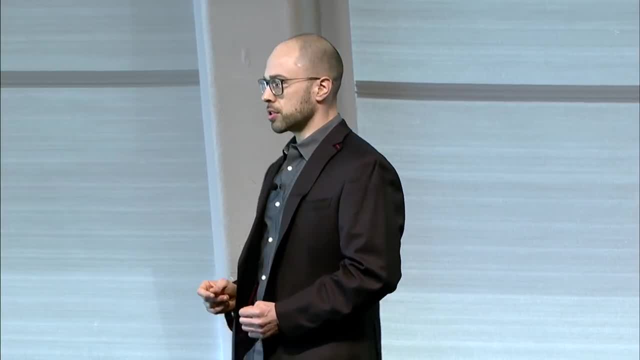 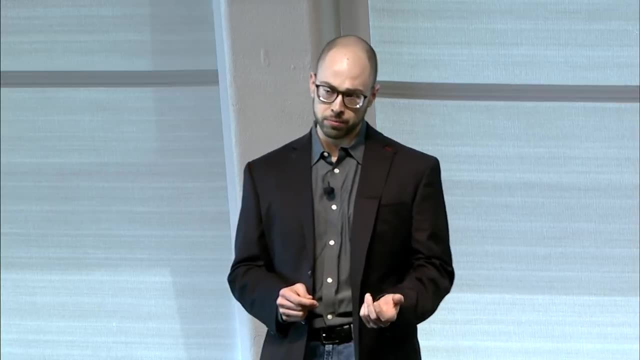 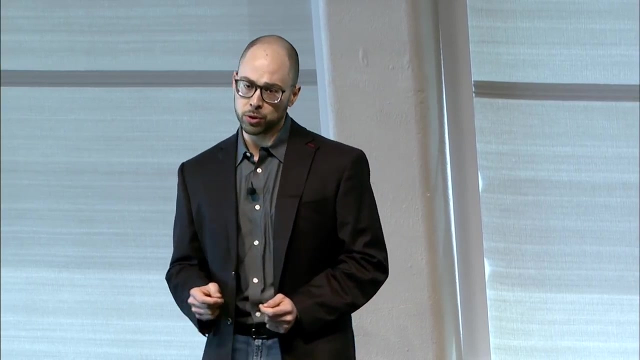 to solve the problems. One in five adults lives with a disability. in the US Between the ages of 65 and 75, that number jumps to one in four Over 75? One in two If disabled. the unemployment rate approaches 70 percent. household income drops by 40 percent. and the poverty rate shoots up by two and a half fold. We are three times more likely to have heart disease, stroke, diabetes and cancer. It all sounds pessimistic, But let me tell you the upside of living in 2018.. 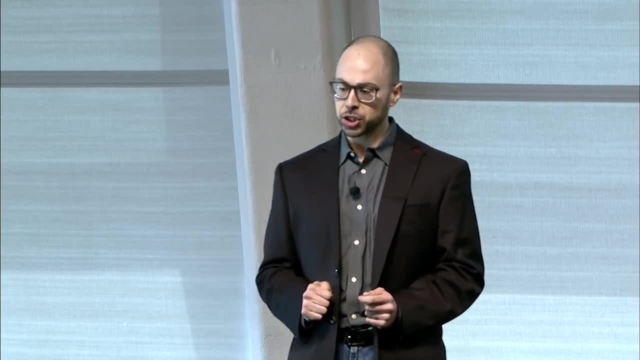 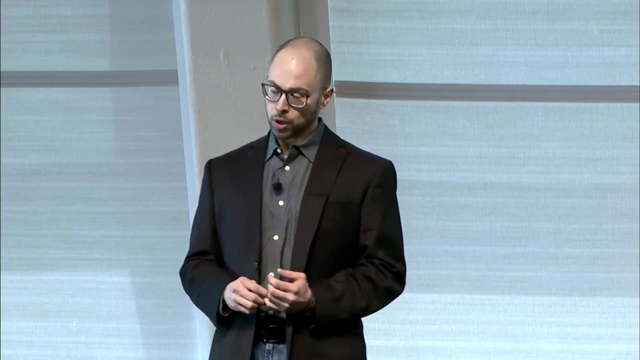 We are now in the fourth industrial revolution, the age of intelligent machines and technology is leaping forward at a measurable speed. You see, I see a different future for us, One where we level the playing fields and destroy previously established ceilings, creating 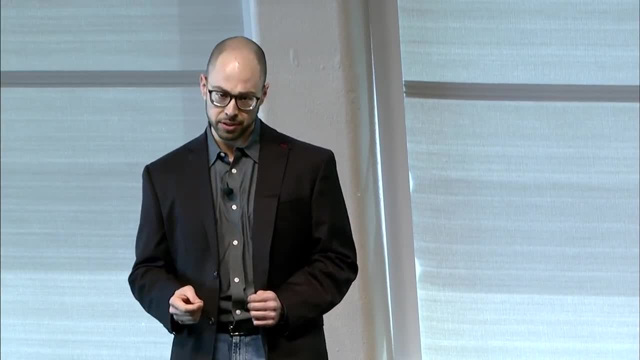 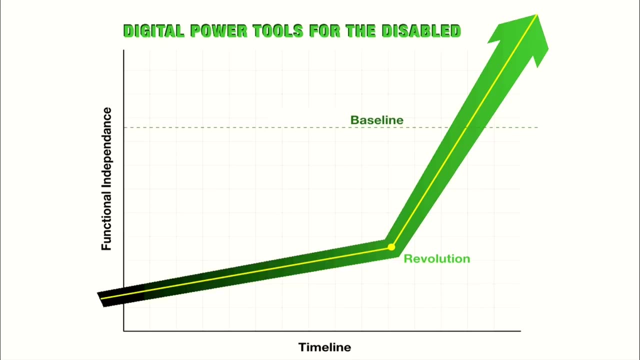 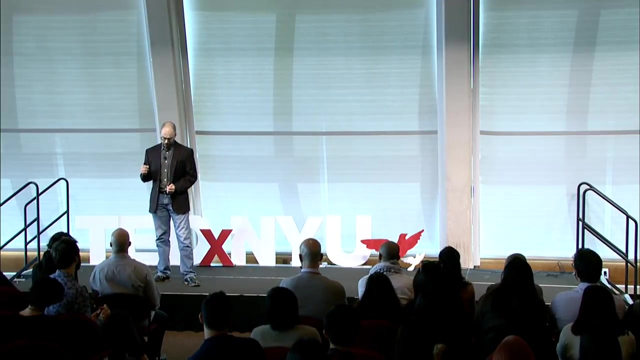 digital power tools that can fill gaps for those in need with disabilities, Tools that not only achieve baseline functional status but that surpass it with new super-abilities. Now I know what many of you are thinking: Is this guy reading too many comic books? 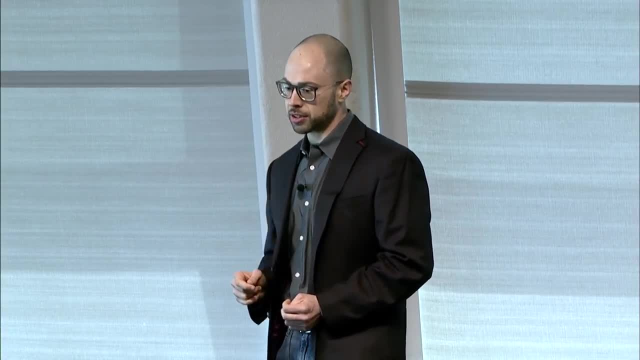 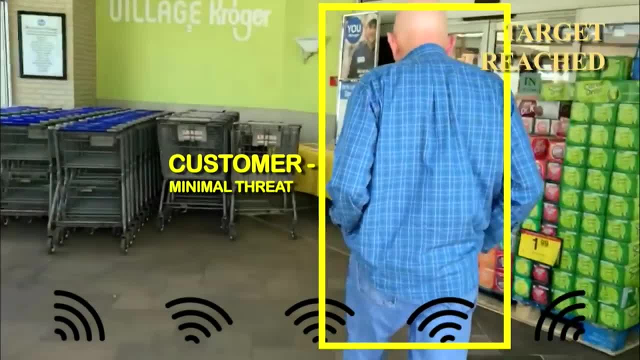 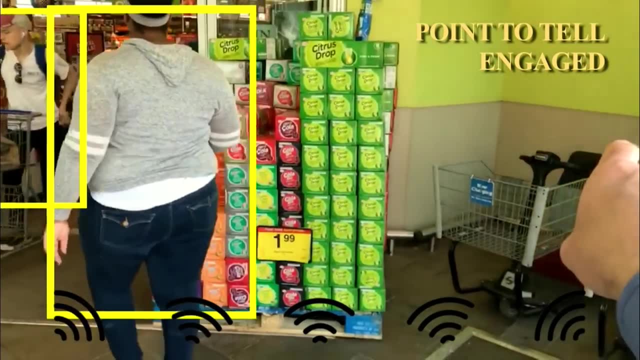 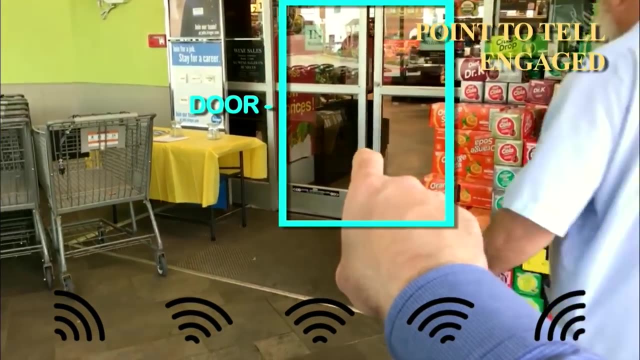 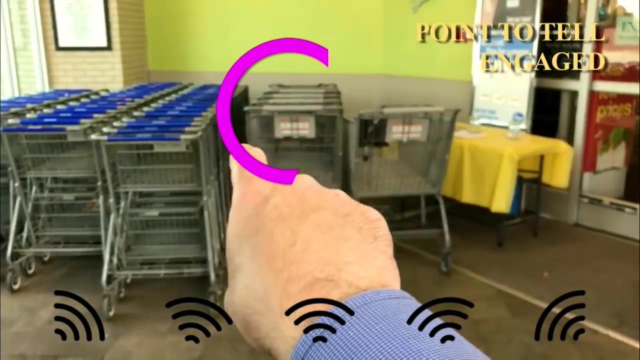 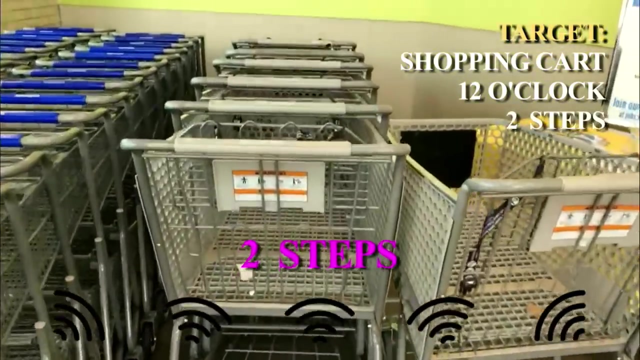 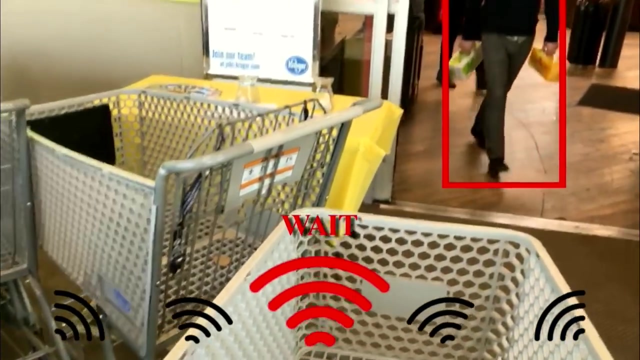 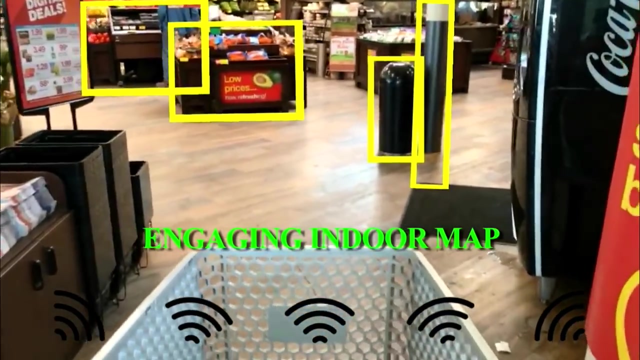 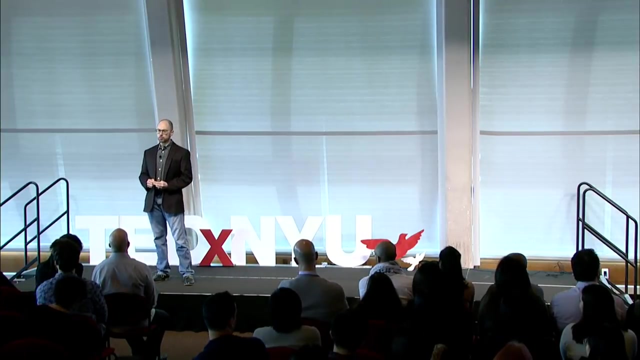 Our video runs in a shorter than 60 target in five steps: four, three, two, one. wait to proceed, customers exiting, wait to proceed, proceed. engaging indoor map, low shopping list and you are off. what if i told you we are close to bringing many of these feature sets into reality? 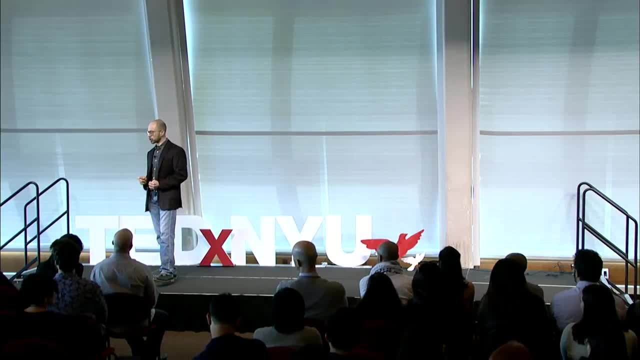 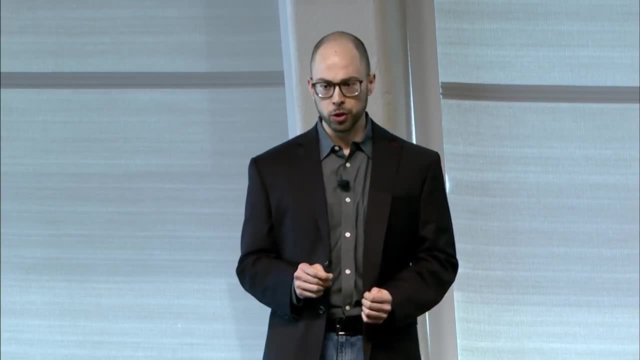 for a wearable. it sounds futuristic, but we have completed the majority of this work in our research laboratories. in closing, i would like to share a few thoughts. disability is a common denominator for the human race race. tearing the d, the i and the s off of disability and focusing on 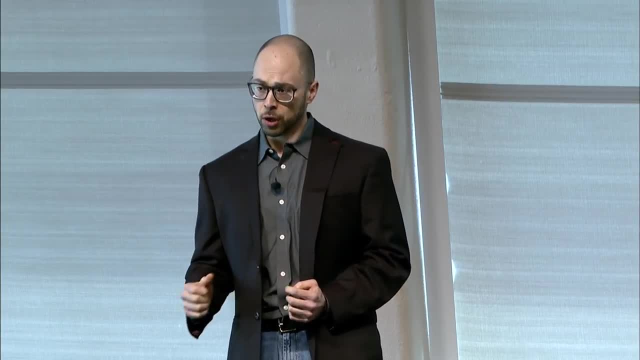 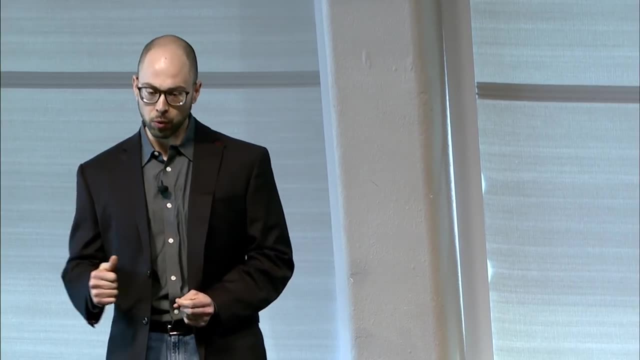 ability is evolution. with new tools, we make the inaccessible accessible, we make the excluded included and we ensure inequalities reverse into equalities. we are now able to unlock the true superhero in the world of the future. we are now able to unlock the true superhero in the world of 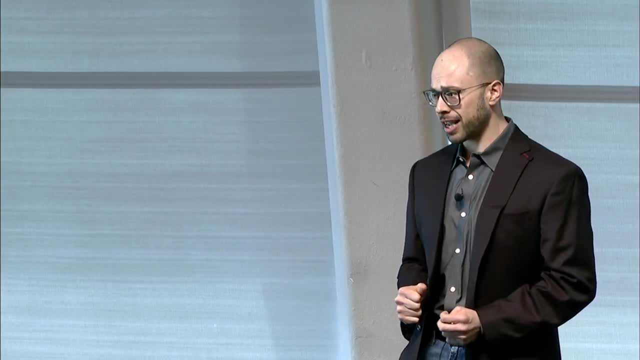 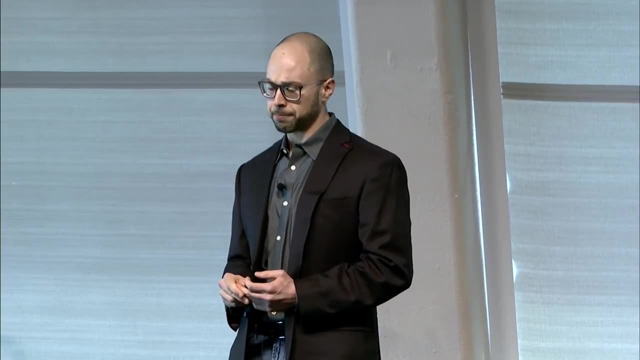 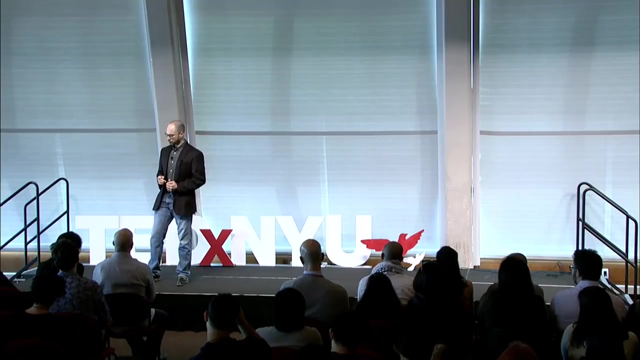 those with disabilities at unprecedented speeds, and with some damn cool superpowers at that. i challenge us all to evolve, channel your frustrations into gains, make shape, invent and rewrite, jump hurdles, tear down barriers and blast through walls. many thanks to you all.